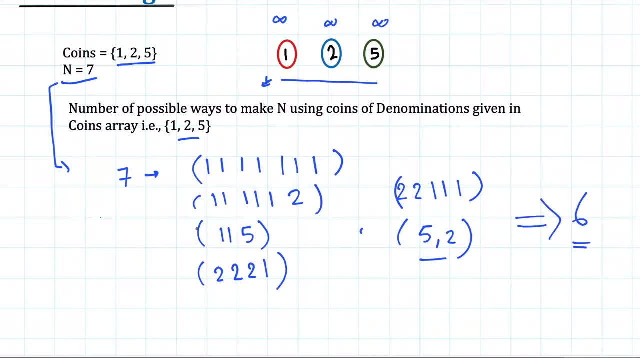 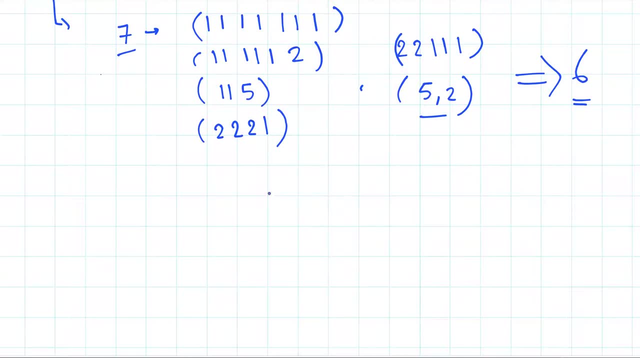 have these six ways of making seven cent using these three denominations of coin. so how can we solve this problem? so we have, we can break it into smaller pieces. we are given the required value and the array of coins: one, two and five. so this is the final problem that we have to solve. 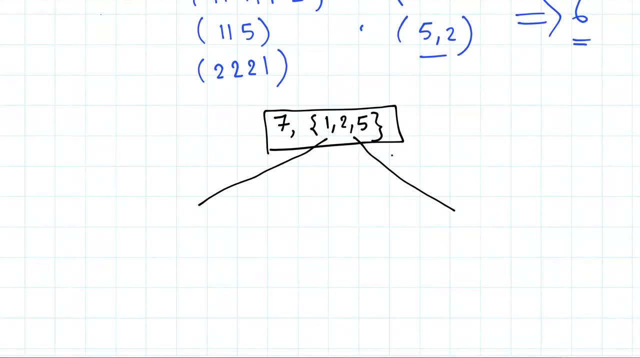 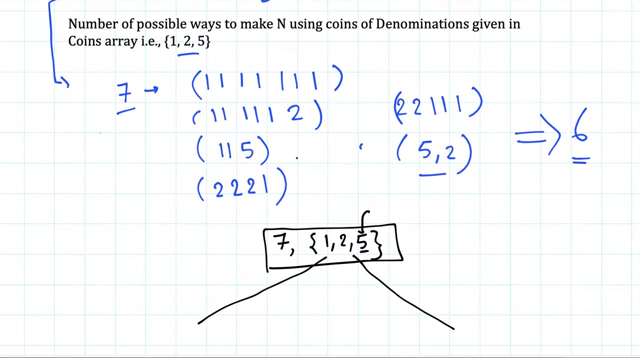 so we can break it into two pieces. so one way would be that i don't include this last coin. so five is the last coin, so i just exclude that. so in my solution does not contain this. so, for example, five is present in this and this and the others force. 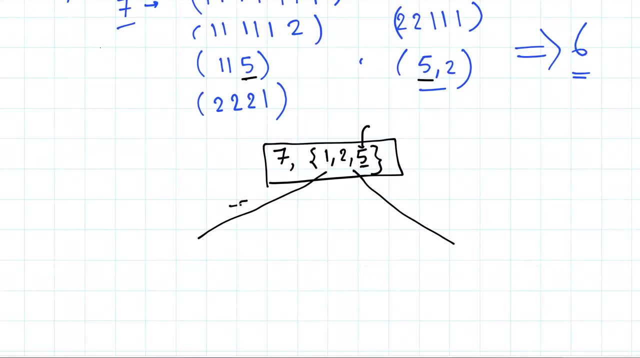 five is not present, so this is minus five, that is, we exclude five. so our problem is reduced to seven and this one two. so this is the same problem, it's just we put the condition that we will not include five, and in the other case we include at least. 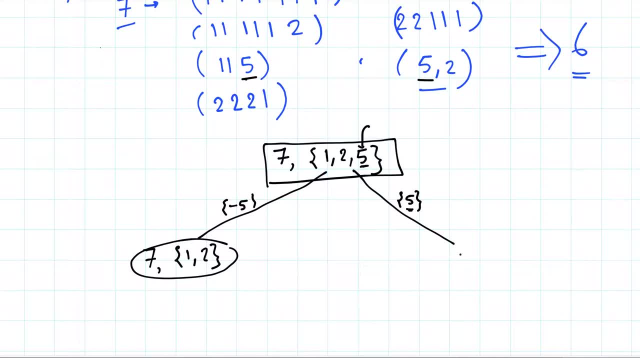 one coin of five cent. so if we include at least one coin of five, then this: we know that one of the coins is five. we have to find the remaining uh possibilities. so our problem reduces from seven to two, because one we have taken five, so now remaining is two and we can use the same set of 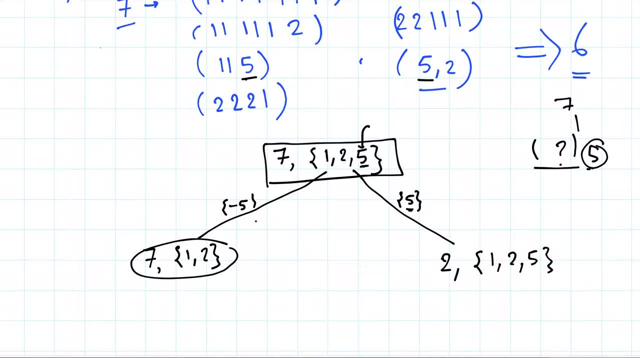 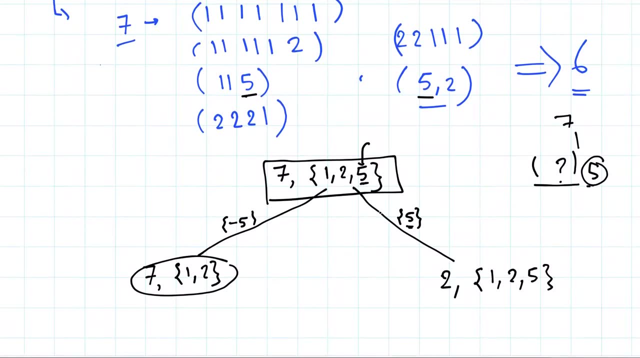 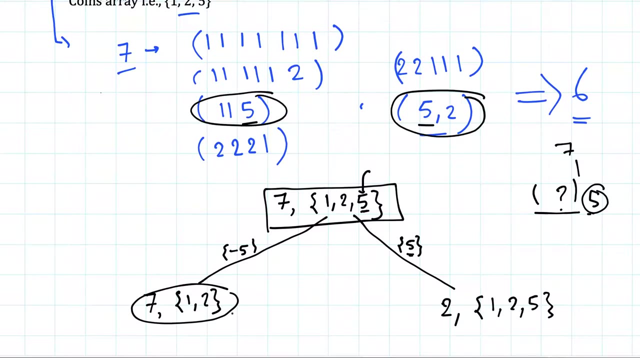 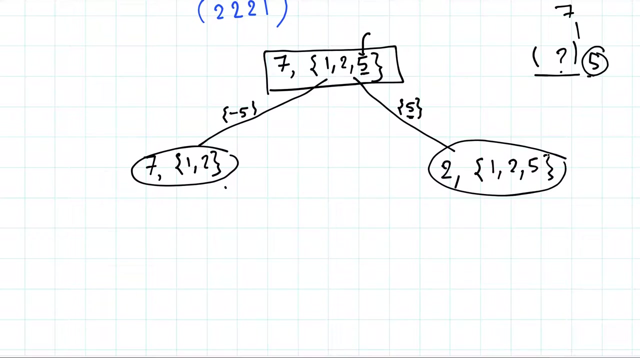 coins. here we had x exclusively said that we will use the same set of coins. here we had x exclusively said that we will exclude five. we will not add five. so this right branch will correspond to these solutions and this left branch will correspond to these four solutions. now we have to break it further and let's define also the base case, like if: 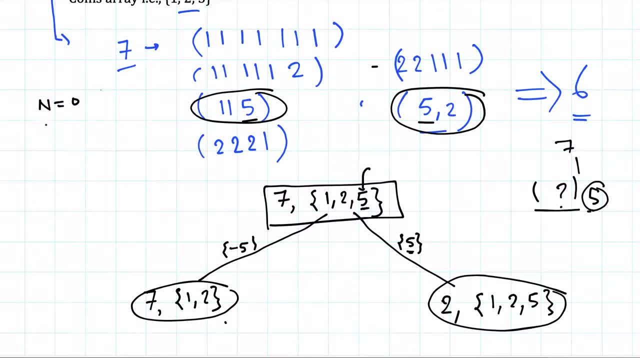 n is equal to zero, then count is equal to one, because if we have to make zero, we will do it in just one way, by by not choosing any of the coins. this is the only possibility. so if n is zero, we will say count is one, and if n is greater than zero but this coin array is empty, then in this case solution would be: 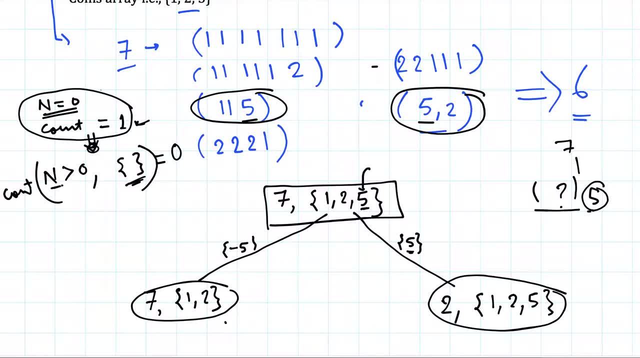 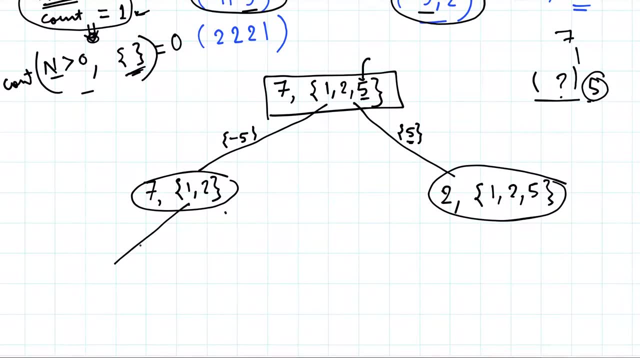 zero, because there is no way to make n without any coins. so we have defined our base cases. now let's break this problem further. so one would be with with excluding this last coin. so we exclude this two. so we have the same problem, but we have to use just one. and in the other case, 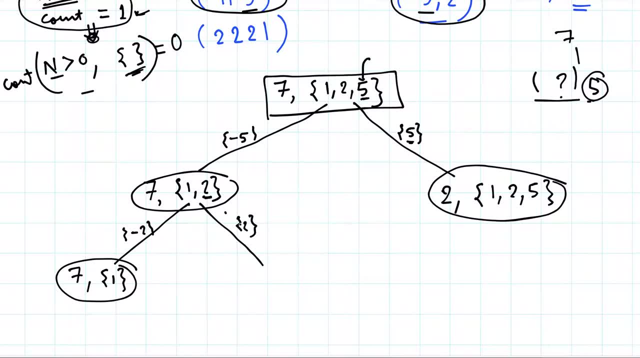 we choose at least one of 2, so our problem reduces to 5 and 1, 2, and now we will exclude this last coin, 5, so our problem will be 2 using 1 and 2, and if we we cannot include 5 because here 2 is less than 5. 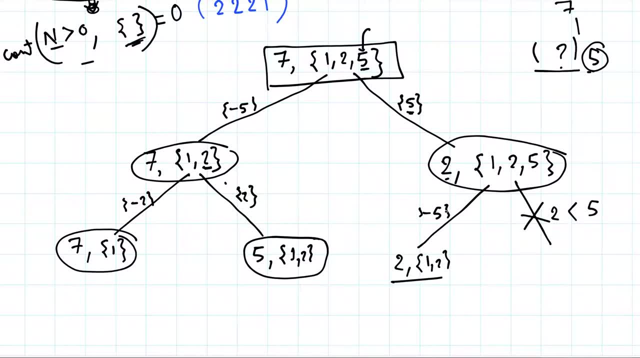 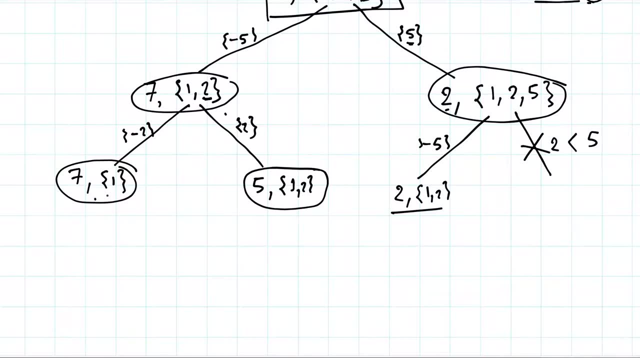 so this branch will not exist, so it will have just one branch. and now, if we have just one coin or one cent coins, either we can go for further and break it into two, like 7 with empty and 6 with 1, or we can terminate here, so we can. 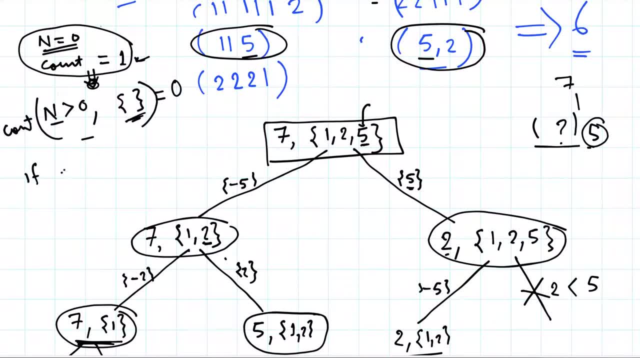 add to our base case that if there is only one coin, then count n should be n. there is only one cent coin and we have to make five or six or seven, then there is only one coin. so we will take it multiple number of times and if it's a factor of this n, then we will have one solution, otherwise zero. 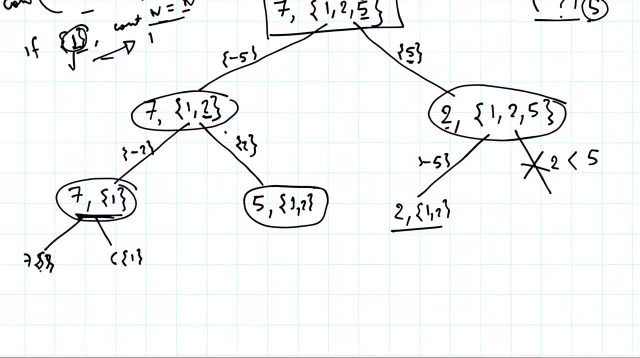 so we could have stopped here also. so here seven, or with empty, this will have zero. so this will return zero. this will in turn call five, one, then one. ultimately it will call one, one and we'll start returning one. so we can stop here itself, that if we reach this case that there is only one, 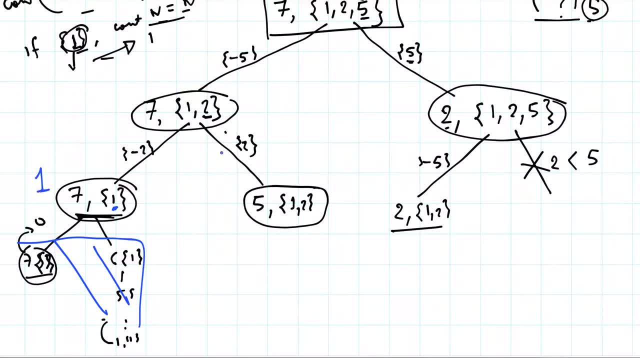 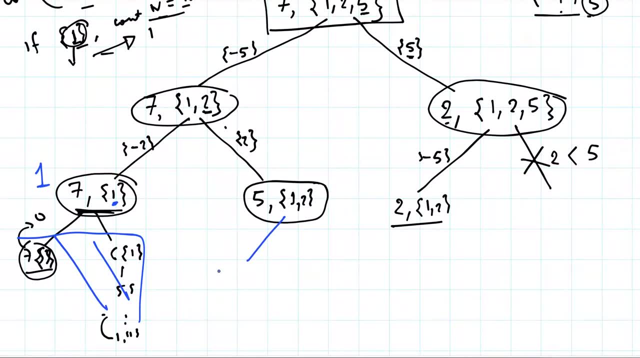 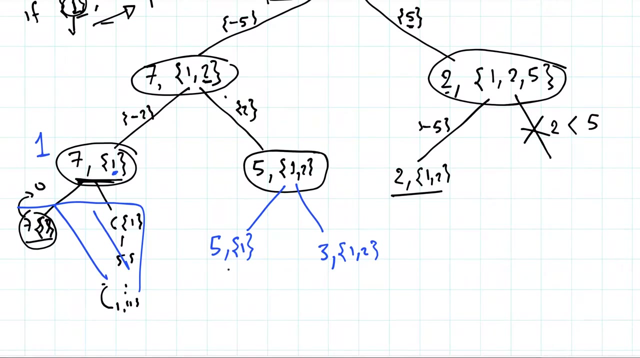 coin, then we will return one, so this has one way. and now we have this 512, so we will exclude 2, then it will reduce to 5: 1 and including 2 it will become 3, 1, 2, and now this will return 1, because again we have reached the base case. and now for this. 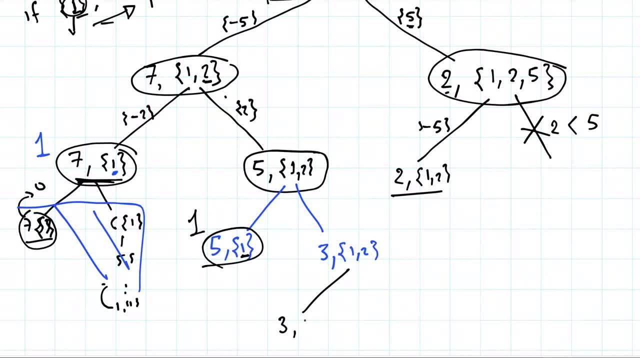 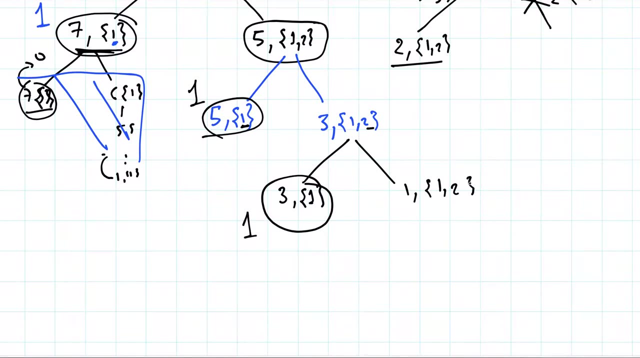 we will exclude 2, so we will have 3, 1 and once we include 2, we will get 1, 1, 2. so this will again have solution 1 and we can break it further. we exclude 2, then we will have 1 and 1 and we cannot include 2 because 2 is more than 1. so this: 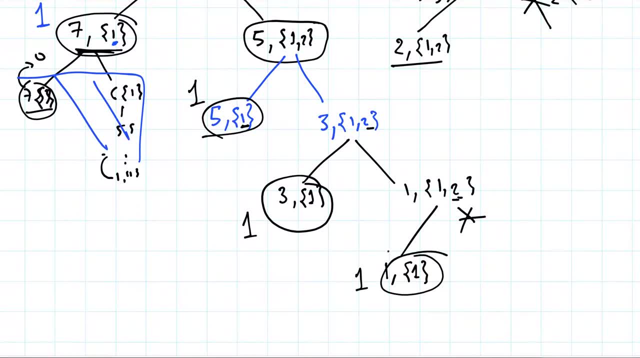 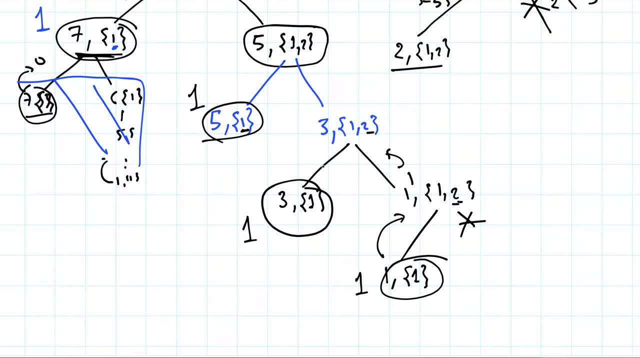 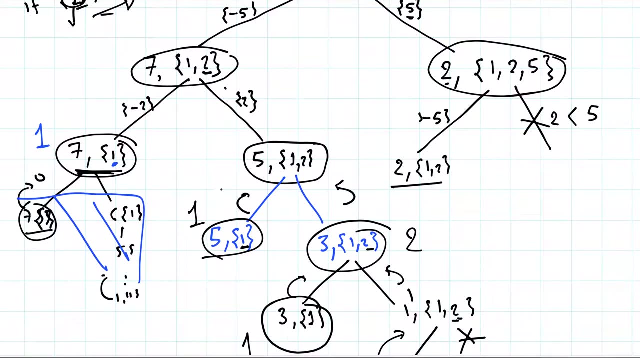 branch will not be there, so this has also 1, so this is 1, so it will return 1, and these both will return 1. so this has 2. now this will return 2. this will return 1. so this has this part has 3 solutions. 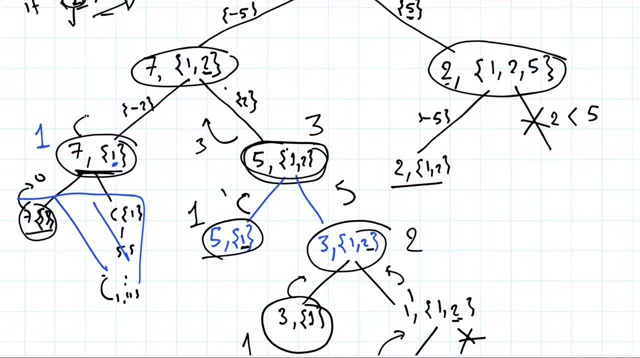 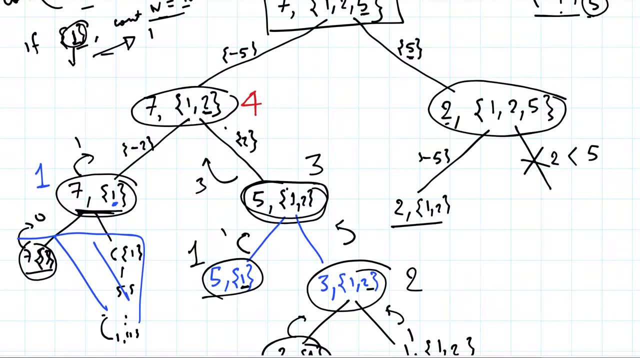 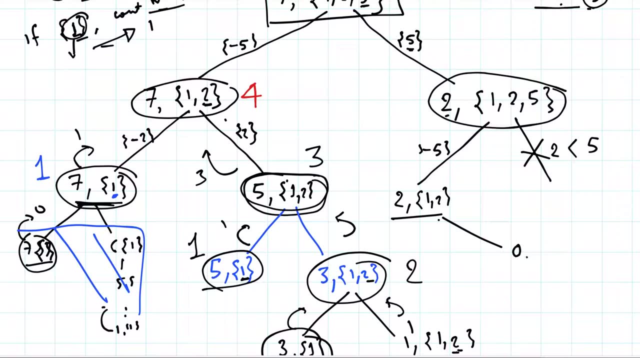 now this will return 3 and this part will return 1, so this will have solution of 4. and now solve this side first. so if we include 2, we will get 0, 1, 2, and if we exclude 2, we get 2 comma 1. so this has solution of 1. 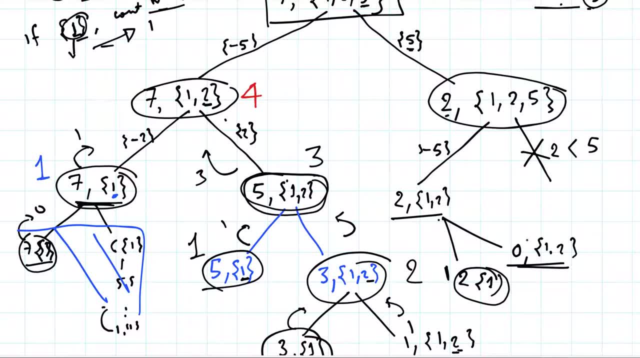 and this. this has also solution of 1, because we have to make 0, so we will not choose anything. so this returns 1. this returns 1, so this has 2 and it has only one branch, because this was not possible, so it returns 2 here. 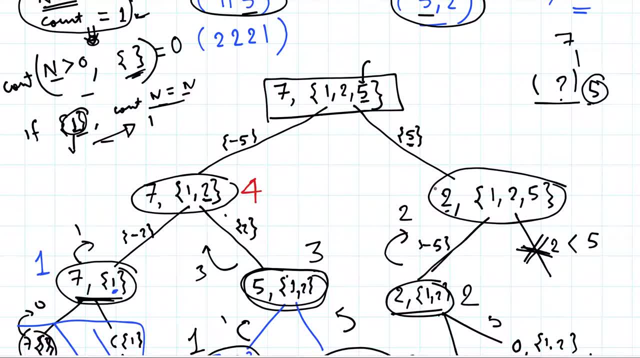 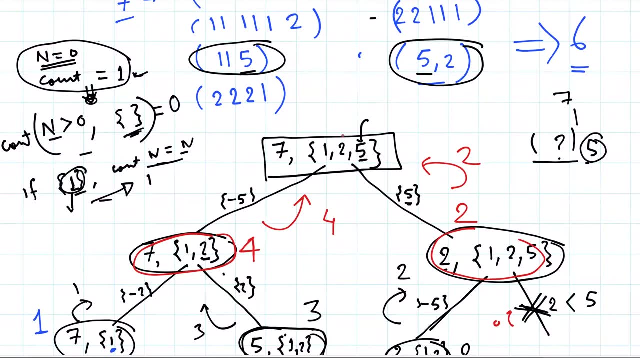 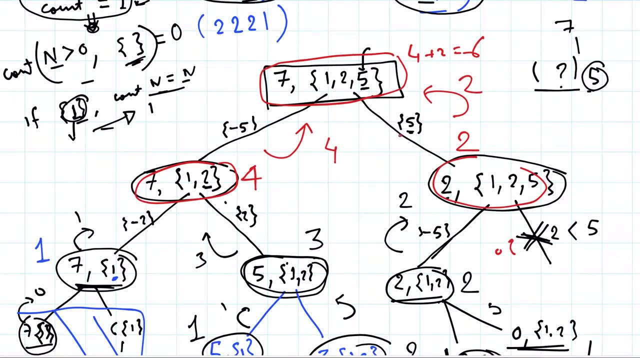 and it returns 0. so this, this part, has 2 and this part has 4, so it will return 4, this will return 2 and ultimately this will have 4 plus 2 is equal to 6, so including 5, we had 2 solutions. excluding 5, we had 4 solutions. 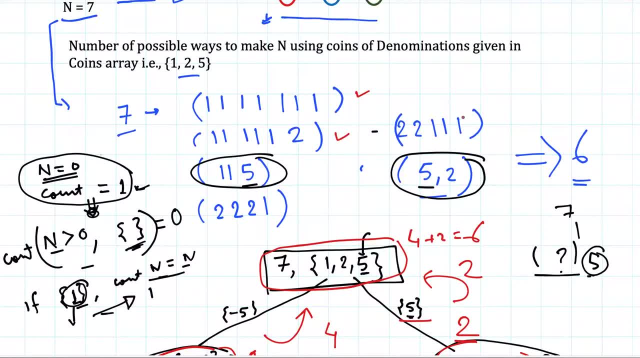 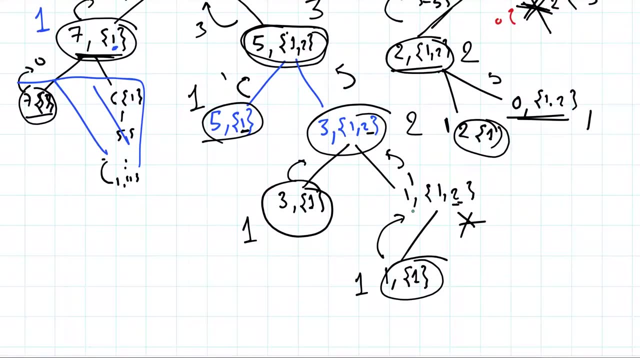 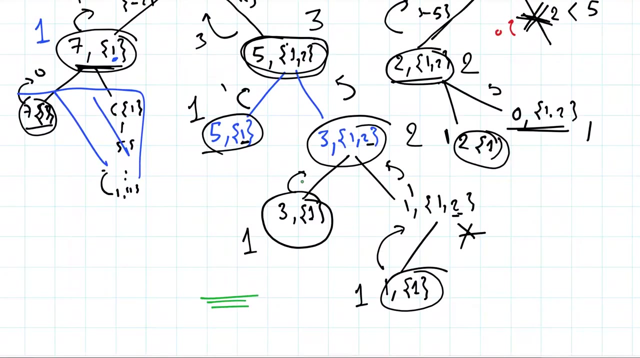 Here you can see that, excluding 5, we have 4 solutions, and including 5, we had 2 solutions. So this exactly matches with whatever we had done manually. So this is the dynamic programming approach, and let's make a table out of it so that it's. 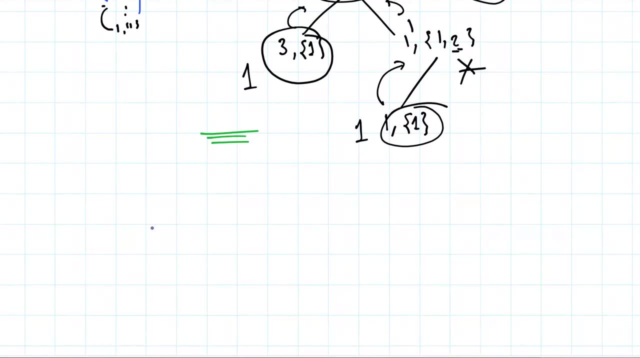 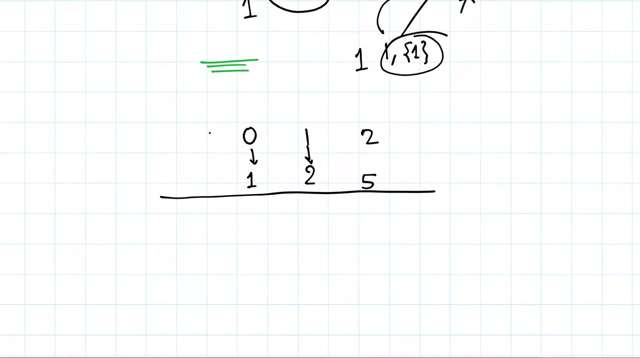 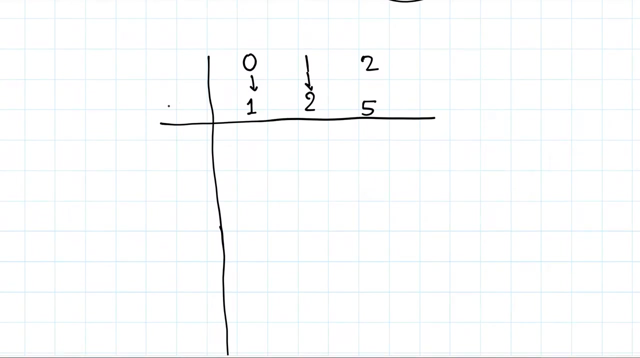 even more clear that how we will approach this problem. So on one axis we can take the values coins. so our coins are 0, 1, 2- these are indices- and at 0 we have coin number 1.. At 1 we have 2 and at 2 we have coin of denomination 5.. 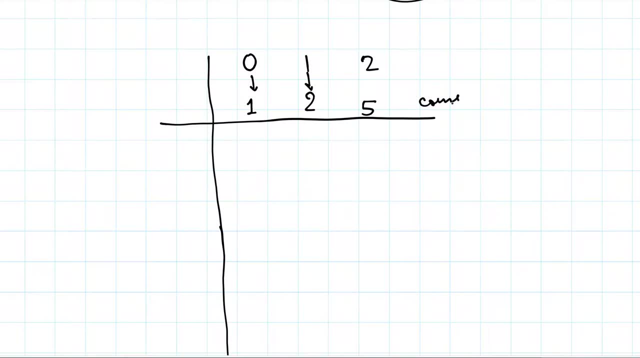 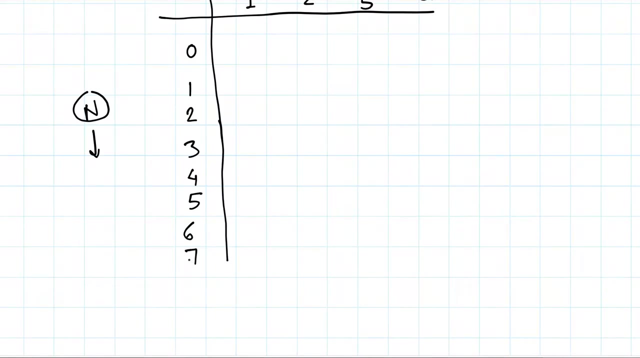 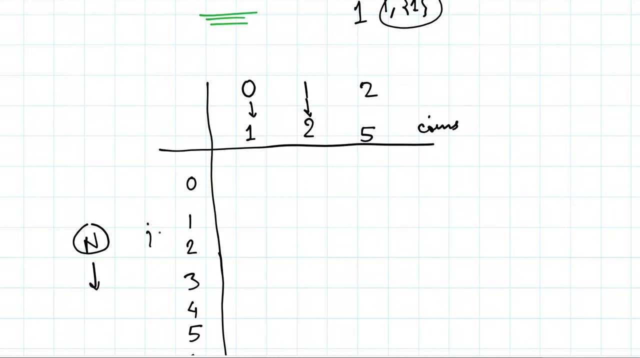 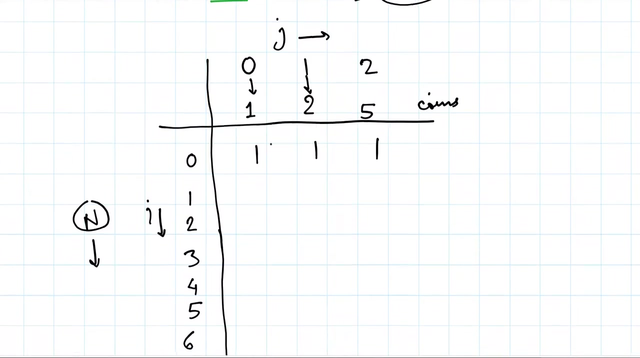 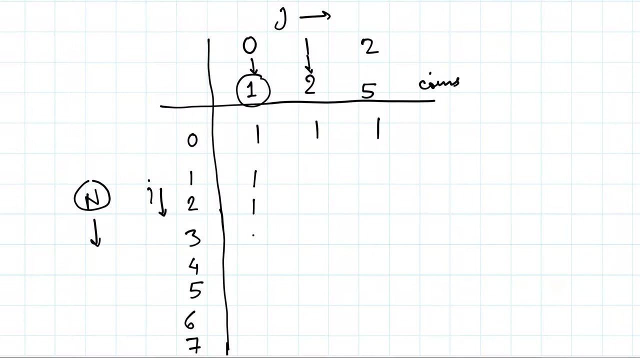 So this is coins. Now we have the values of n, So 0, 1, 2, 3, 4, 5, 6 and 7.. So if we have to make 0, then there is only one possibility, And if we have just one coin of one cent, then also there is only one way: repeat this coin. 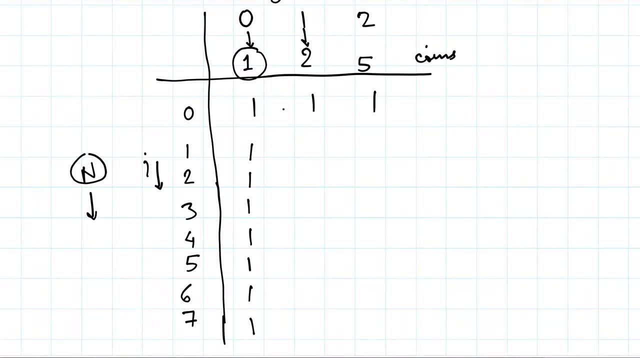 As many times as we want. So we fill this part. Now let's fill this part. So here we have to make 1 using coins 1 and 2.. So this index means that you can use coins till this point, That is, 0 and 1.. 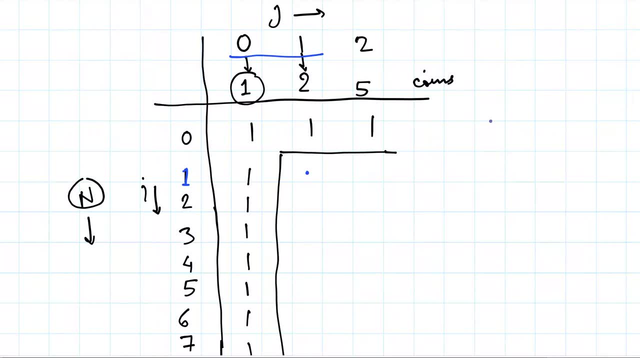 So this is 0 and 1.. And you have to make 1.. So here 1 will branch into two parts, one including this last coin, 2, and the other part excluding 2.. So, excluding 2, it will reduce to 1: 1, 1, 1 case, that is this part. 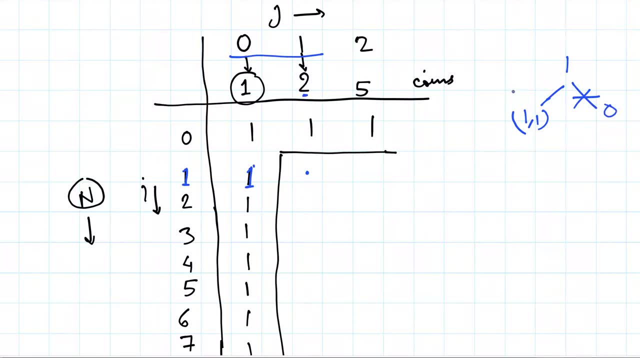 And this, possibly, this is 0, because this branch does not exist. we cannot include 2.. So 1 plus 1.. 1 plus 0.. 1 plus 0 is 1.. And now we have to make 1 using 5.. 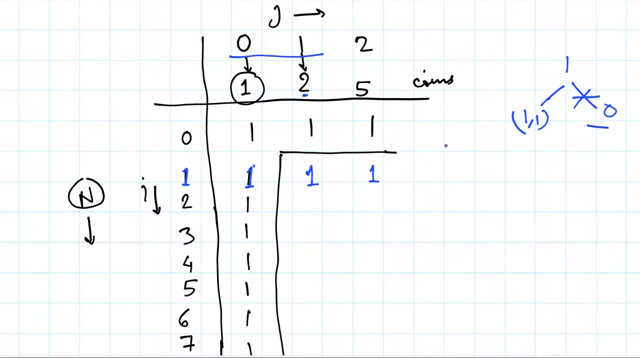 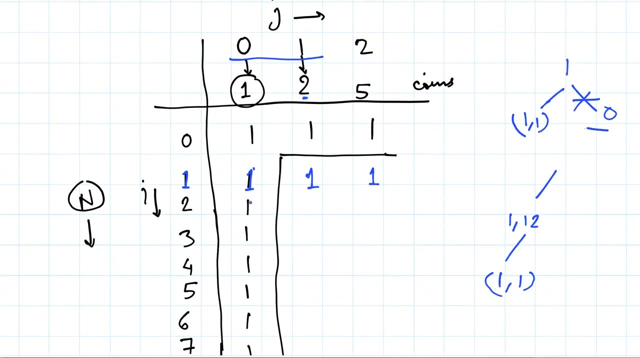 Again, this will be 1, because second branch will not exist. So it will reduce to 1 using 1, 2 and it will ultimately reduce to 1 using 1.. Now for 2.. So 2, 2.. So we have to make 2.. 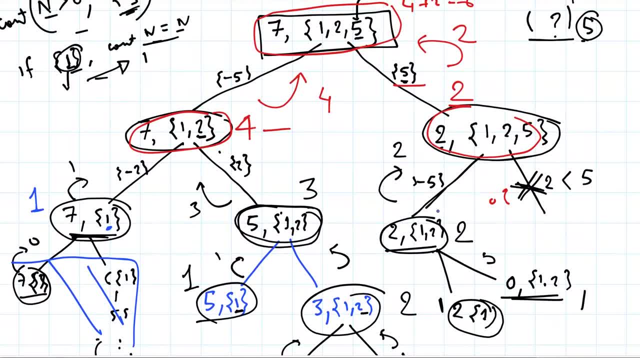 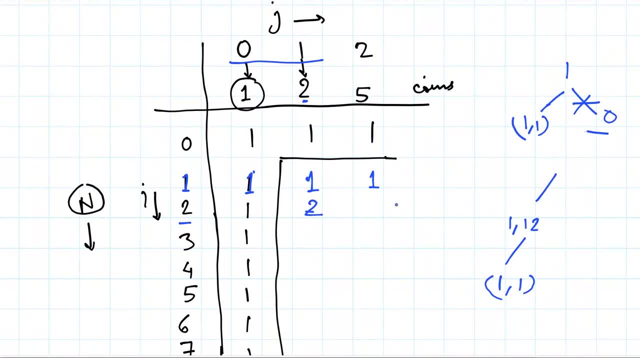 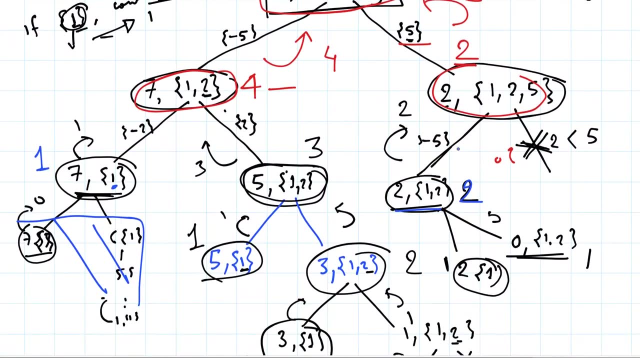 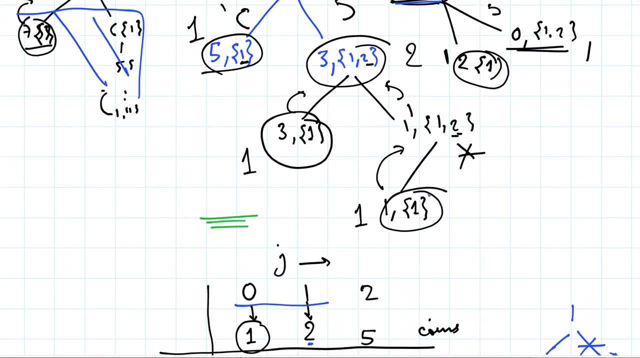 2., 2., 2., 2., 2.. This return 2., So its value will be 2 and then 2, 3.. So some of the part was not used, so it was not completely mandatory, So we can similarly fill for any value. 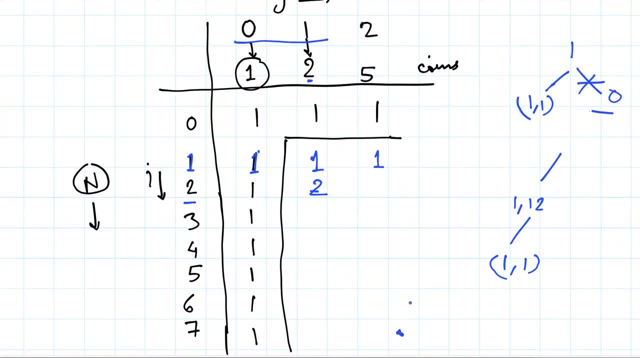 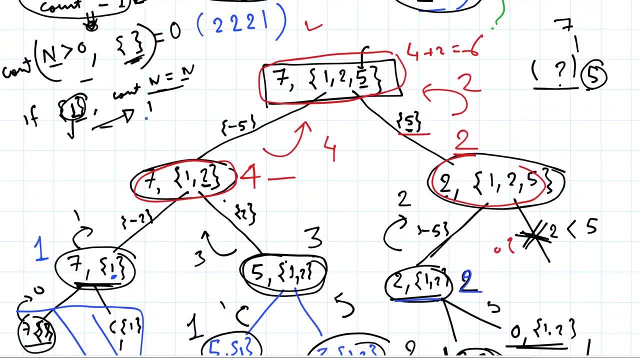 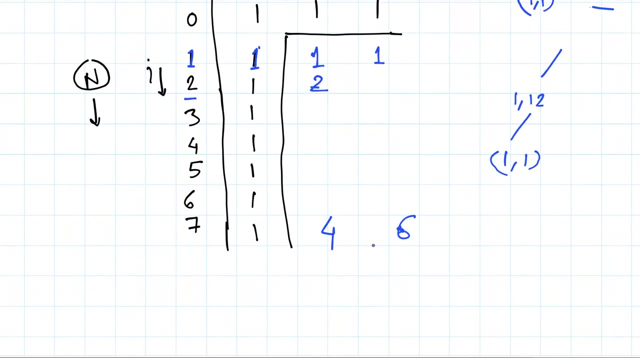 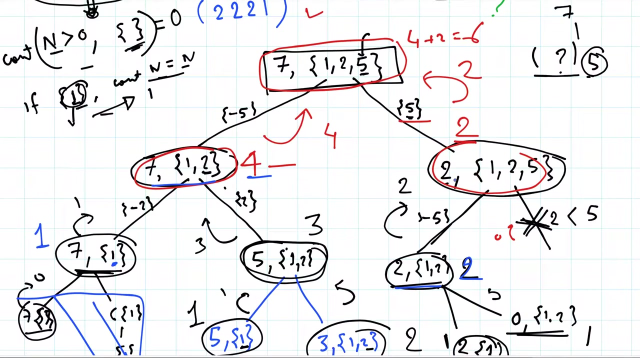 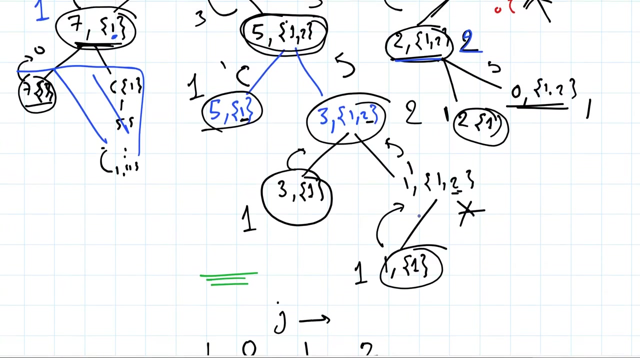 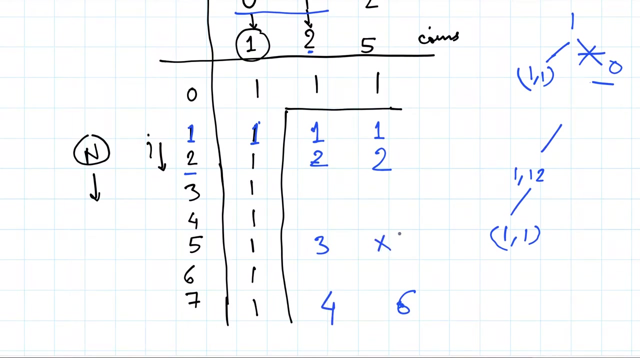 we have to fill here 75. we just calculated here its value is 6. and where did we get that from? we got that from 72, whose value was 4. so this part is 4. now 5, 2, 3 was 2, 2, 3 is 2, then 5, 2 is 3. so for calculating other values also, we can. 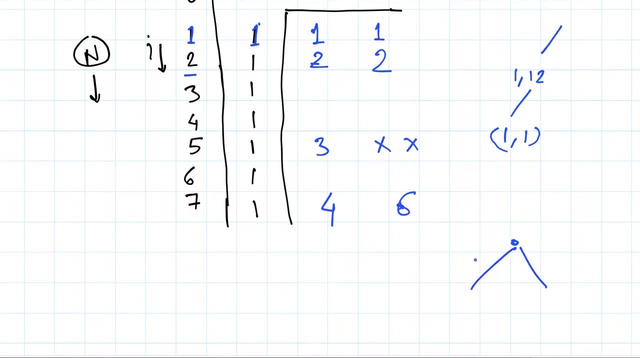 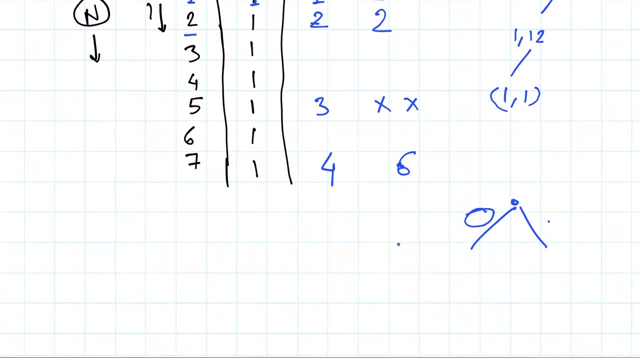 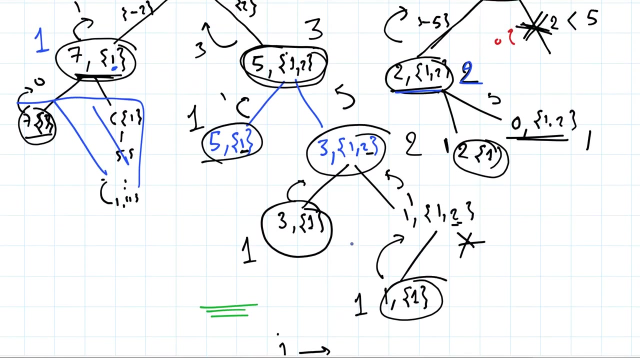 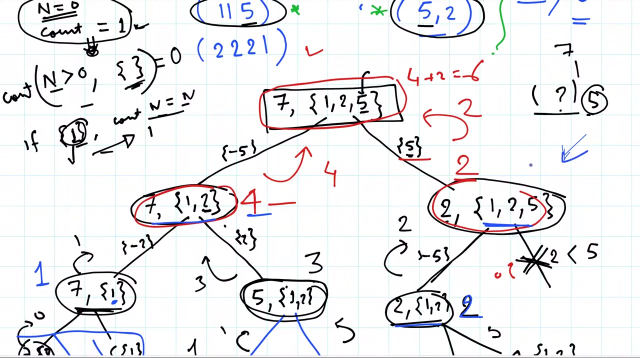 just break it into two branches, one with excluding the last coin and one with including the last coin. so now let's write the code for this. so filling this table would mean resolving this, this recursive tree, so you can try out and find other values. so let's first look at the code. 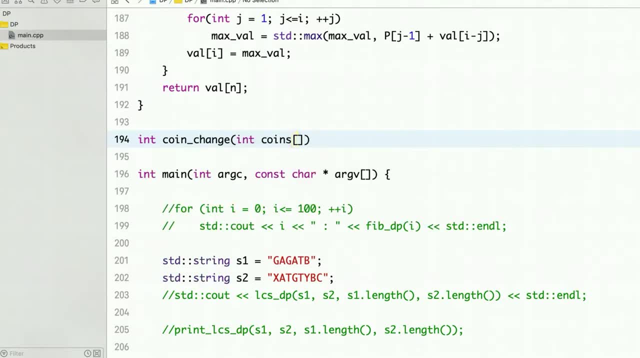 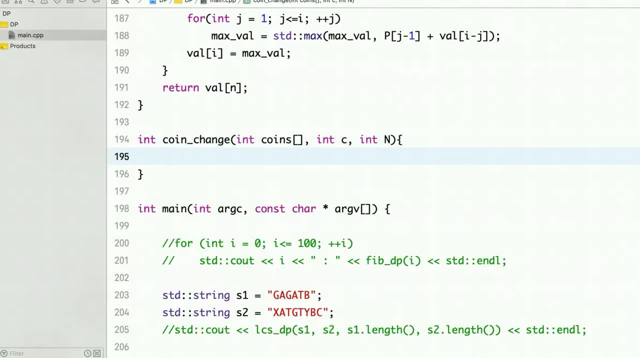 then the size of that array, and then the size of that array and finally the value that we want to make. so we finally the value that we want to make. so we finally the value that we want to make. so we will keep one 2d array and let's name 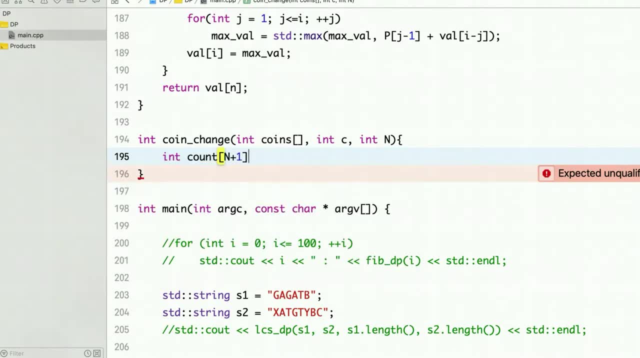 will keep one 2d array and let's name will keep one 2d array and let's name it count switch n plus 1, and see so one. it count switch n plus 1, and see so one. it count switch n plus 1, and see so one extra value because we have to take into 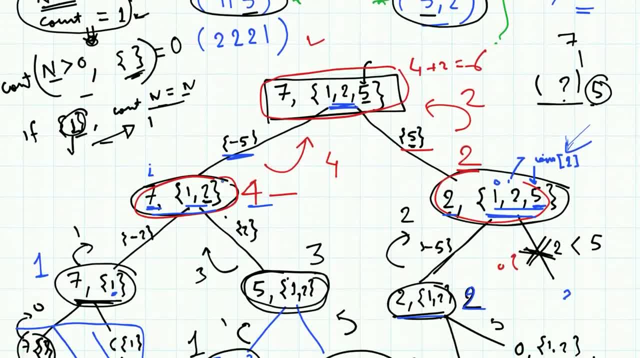 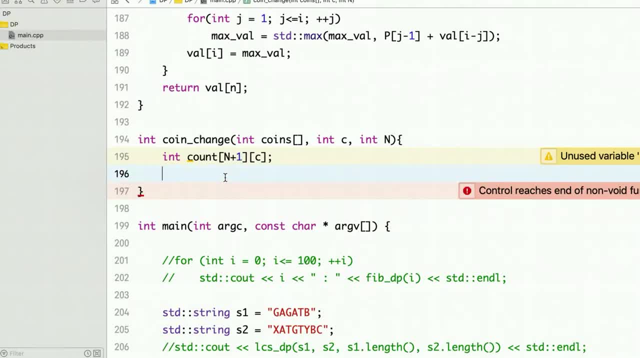 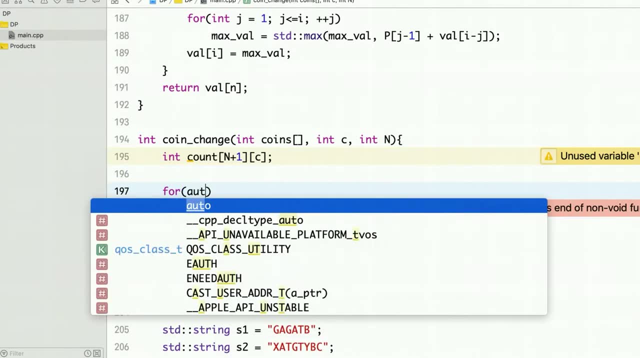 extra value, because we have to take into extra value, because we have to take into account that 0 case also, so this zero account, that 0 case also, so this zero case. so that's why one extra. now we will take two loops corresponding to n and C. 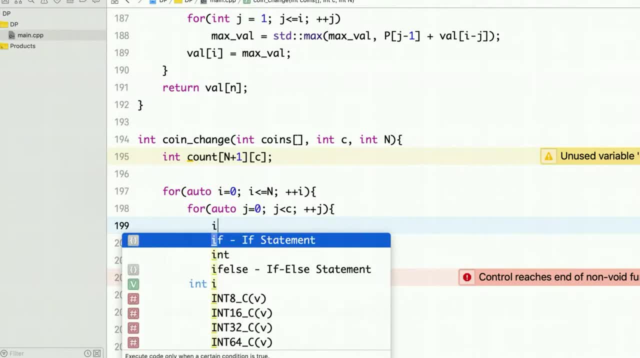 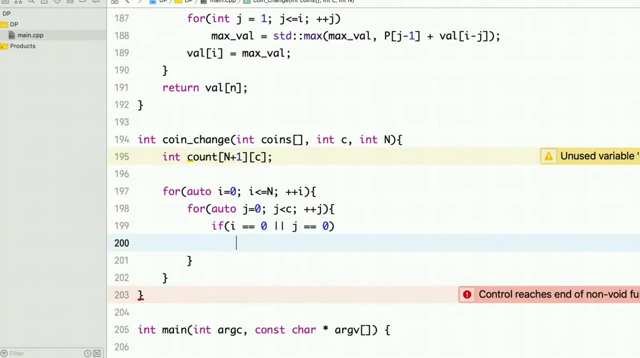 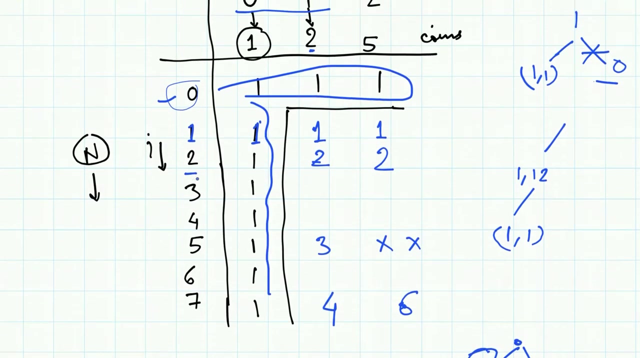 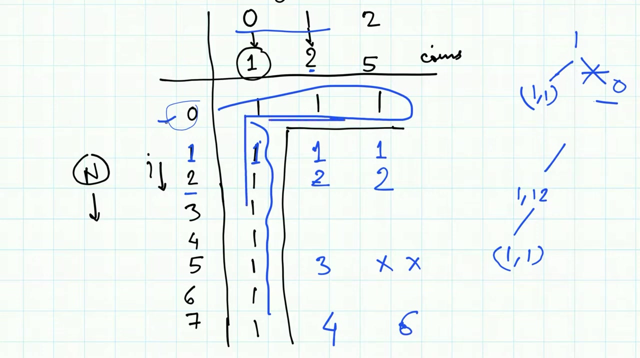 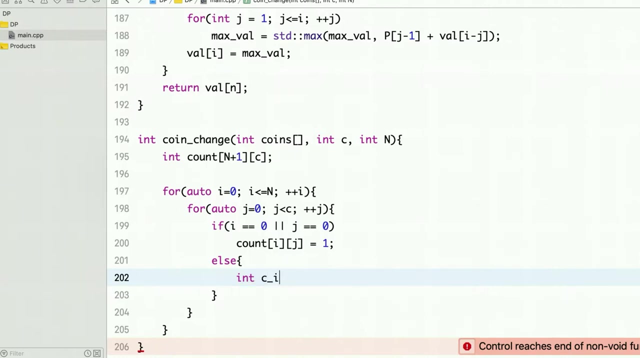 so if any of I or J is zero, then we will simply populate zero, because if this first row and first column is zero, so if I is zero, then also everything is zero. if J is zero, then also everything is zero. else we will have two values, one including C. so we include only when this I, so here inside. 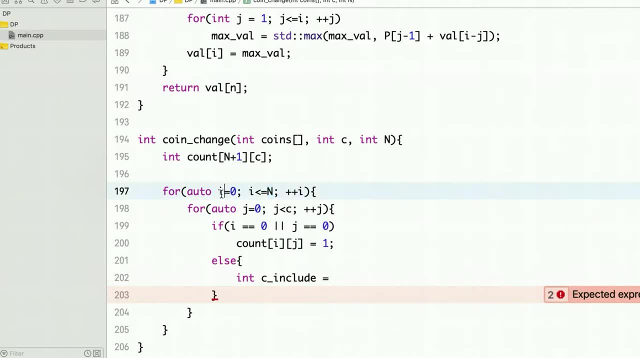 this loop. so n is the final value that we want, but inside this loop I is the value that we want to generate using coins from indices zero to J. so if I minus coin at index J is greater than equal to zero, then only we will include zero. when we exclude last coin, then include that coin, else return zero. add 0 to nat and. 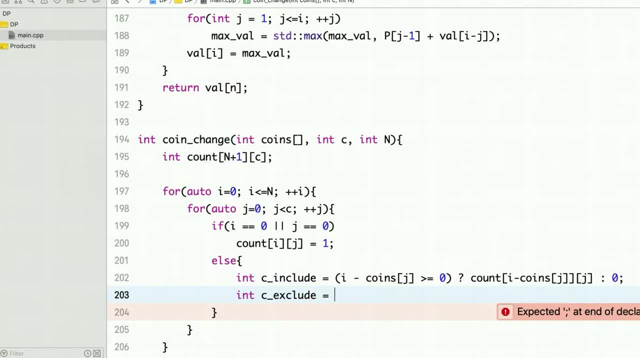 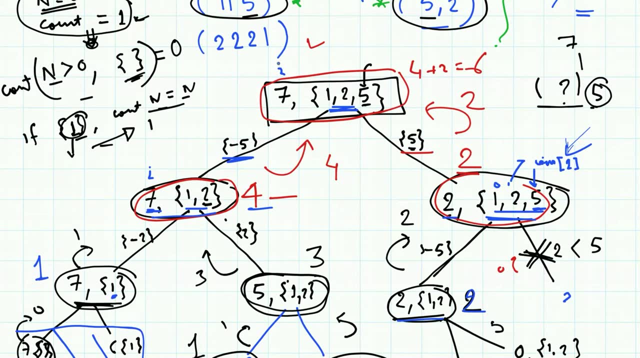 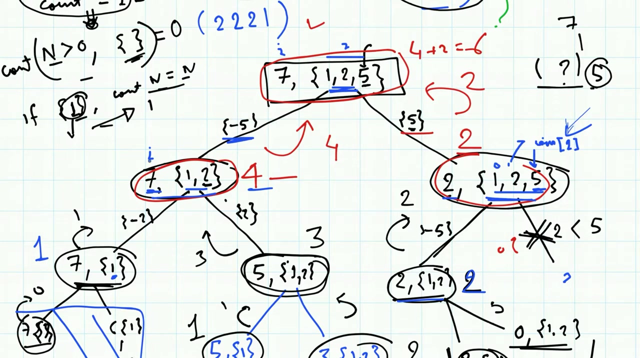 the second would be excluding that last coin. when we exclude last coin, what we do? so this was our initial problem. in this case, I would be 7 and they would be 0, 1, 2, because it has elements, this array, so j would be 2. so if we exclude that, this problem reduces to same. 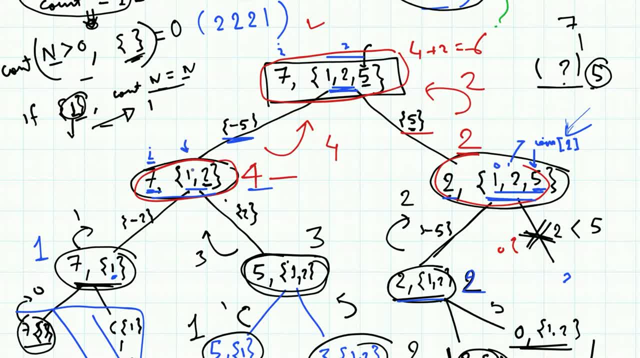 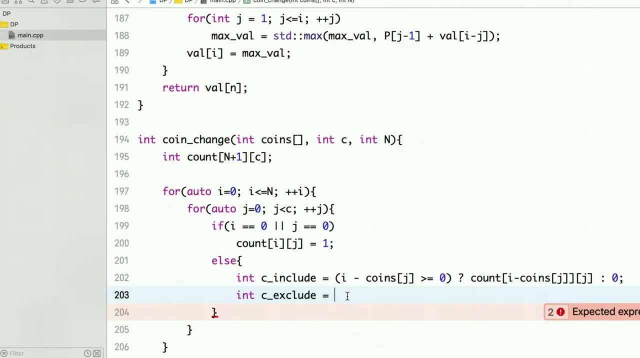 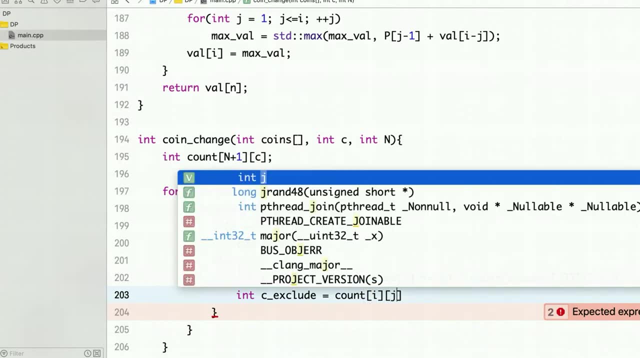 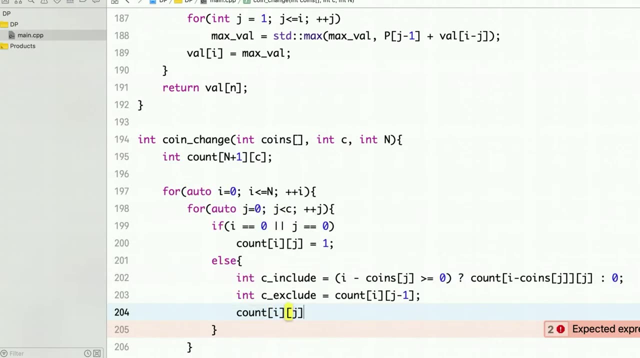 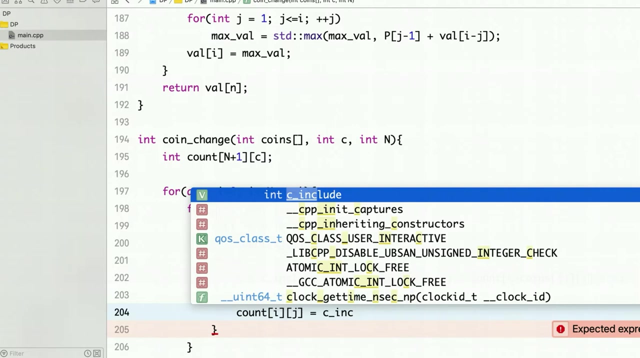 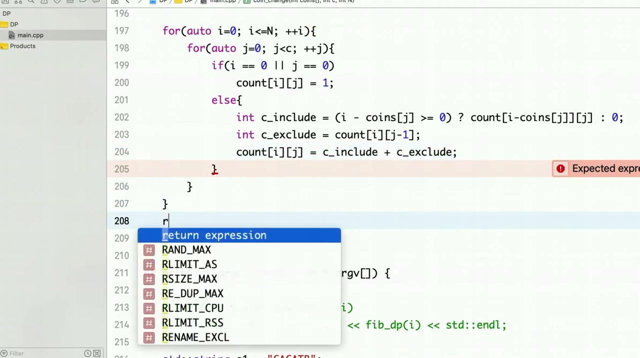 i, but this j decreases by 1, we exclude that last coin. so in that case we will have simply count- i will remain same j minus 1- and finally add these values and populate it in sports array, And then we can return the last element, last value inside the count array, at position n.